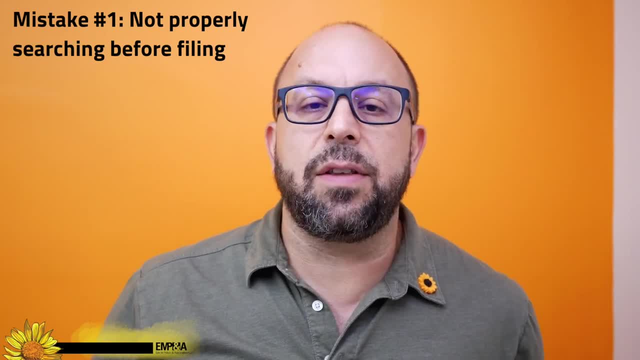 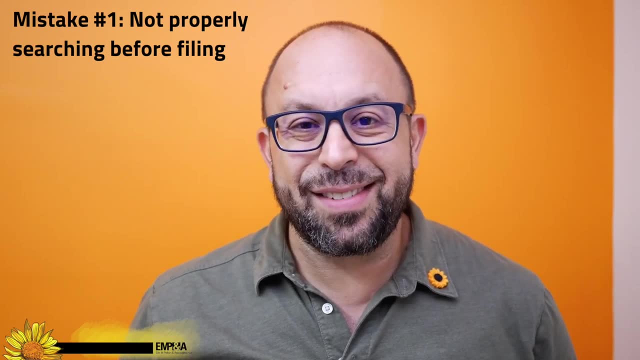 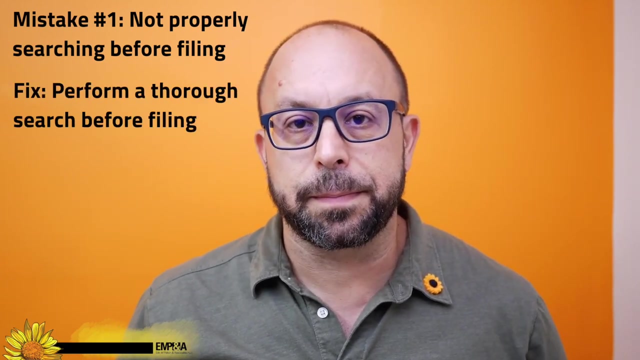 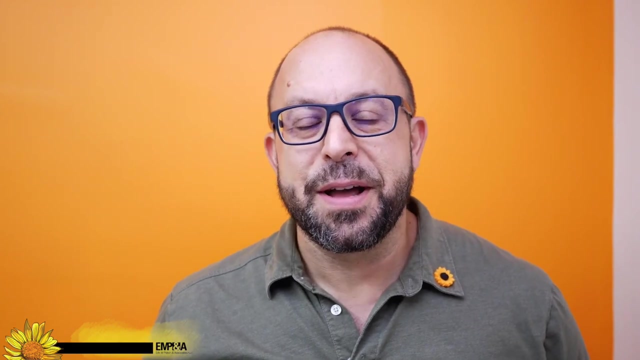 conflicts is a significant factor in the strategy of whether to file and how to file the trademark application. So the way to fix this is to ensure that a trademark application is not a search is done before a trademark application is filed. a second common mistake that we often see is those who dilly dally or wait before they're filing. 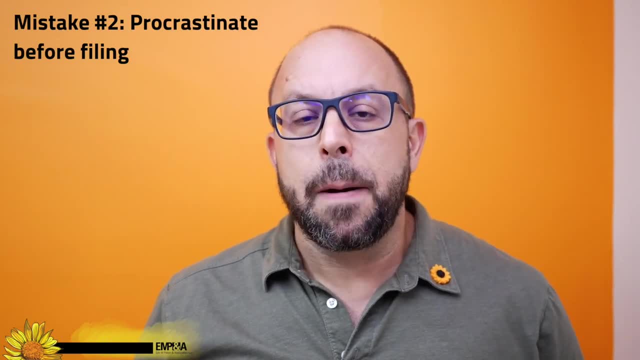 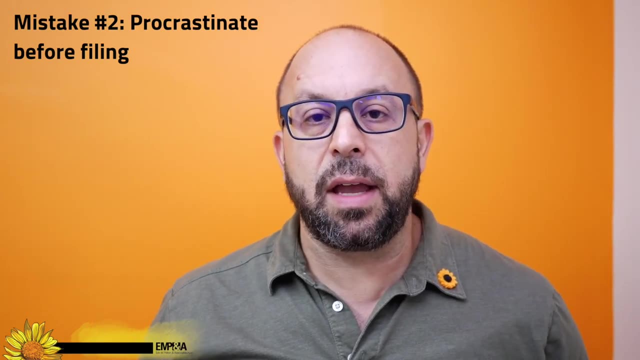 They might think about filing and then hold off for some reason. The longer you wait, the more exposure you have as a brand owner or as someone launching a new brand, because in the end you're not going to be able to achieve the outcome of your job. in the end, you're not going to achieve the outcome of your job because in the end, you're not going to achieve the outcome of your job. So when you're firm with your brand, you go to yourWORK, you're going to go to your agency, you're going to go to the agency to mark a landmark. 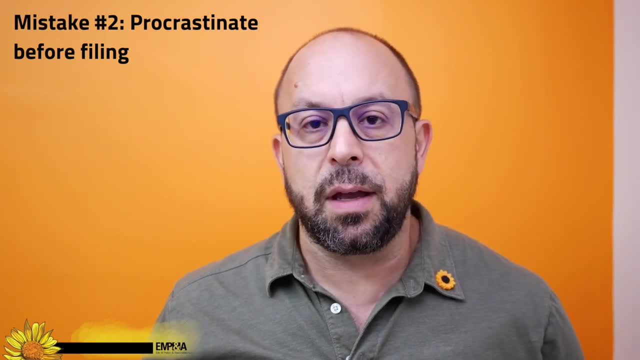 So you want to be a part of it, You want to be the part of it, You're going to be the part of it And then you're going to take care of your business In the interim. if someone else files something that could be confusingly similar, it is likely. 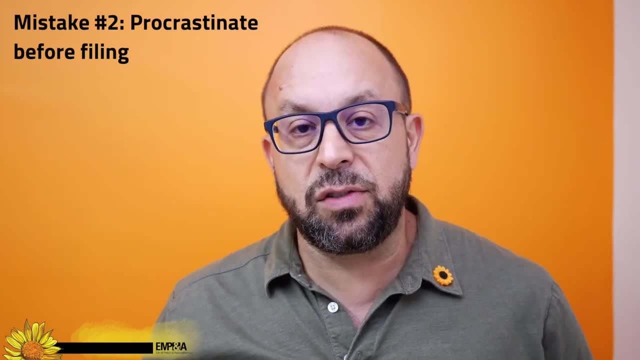 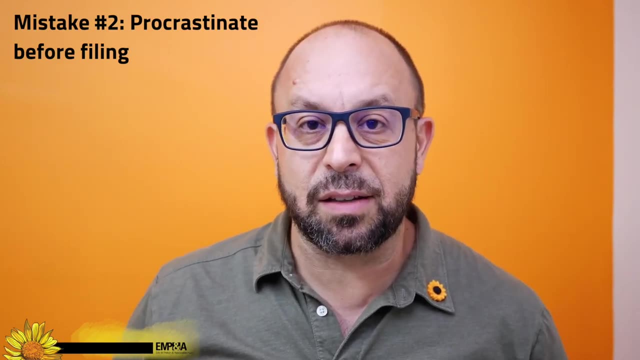 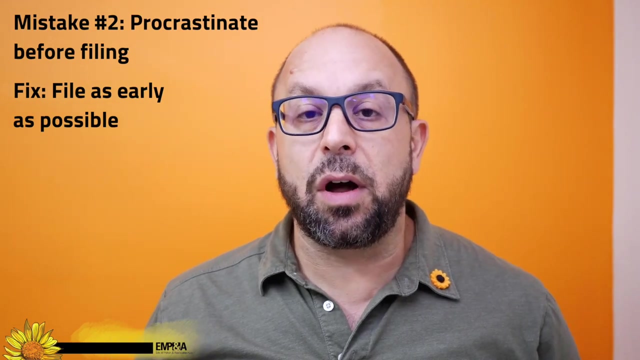 to cause problems, delays, expenses or refusals or some combination of all those things. This is also a relatively easy fix. The answer is to file as early as possible. Applicants can file based on intent to use the trademark before they're actually launched. 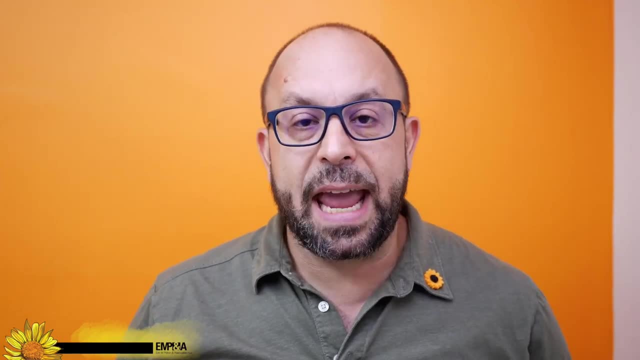 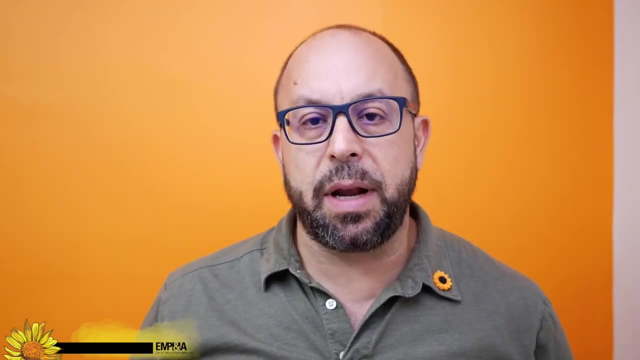 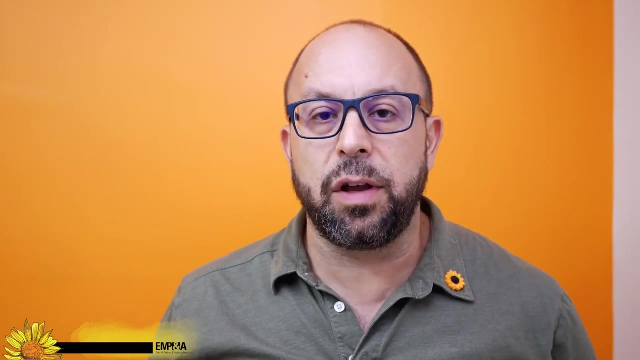 and using it in commerce. And once they're using it in commerce, they can and should file as soon as possible in nearly all circumstances. A third common error that I see over and over again is not fully understanding what use in commerce is and what the requirements are for that. 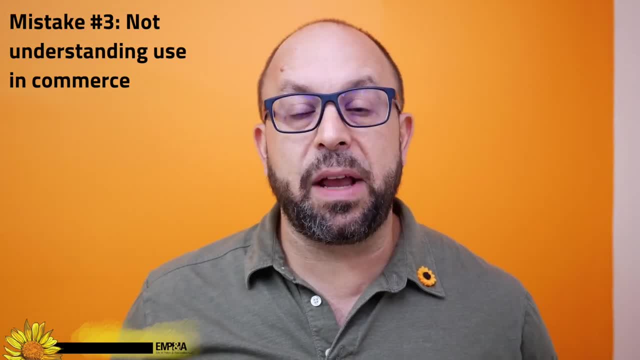 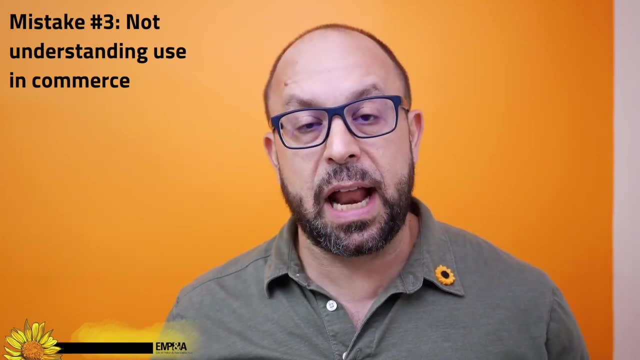 As I mentioned a moment ago, it's possible to file an application based on bona fide intent to use. So use in commerce isn't required at the outset, but it is required in order to complete an application, No matter what, with some exceptions for foreign filings that I'm not going to get. 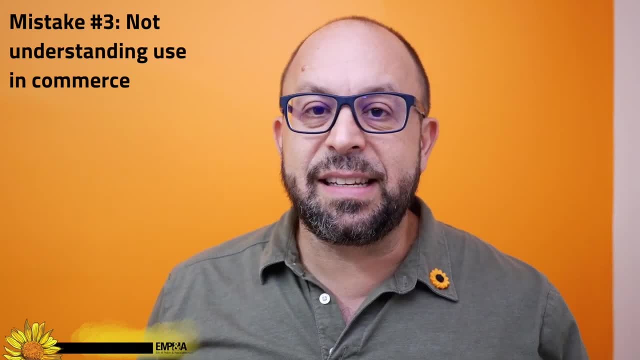 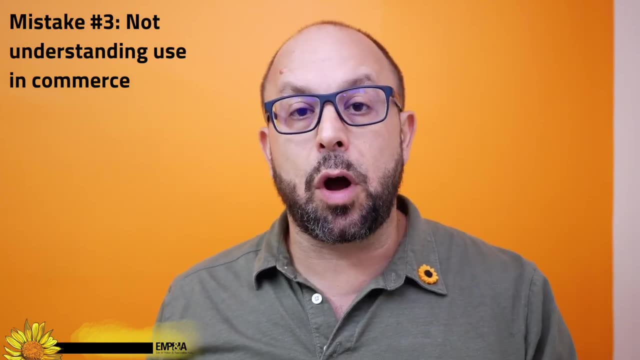 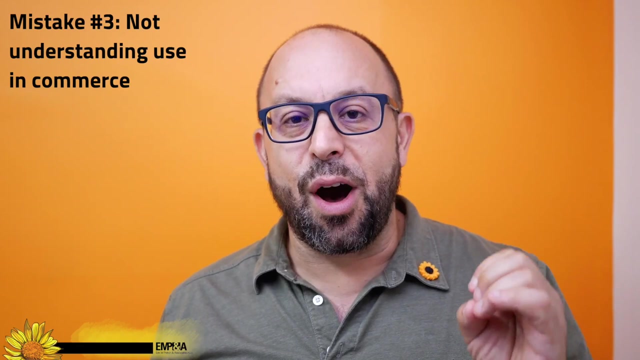 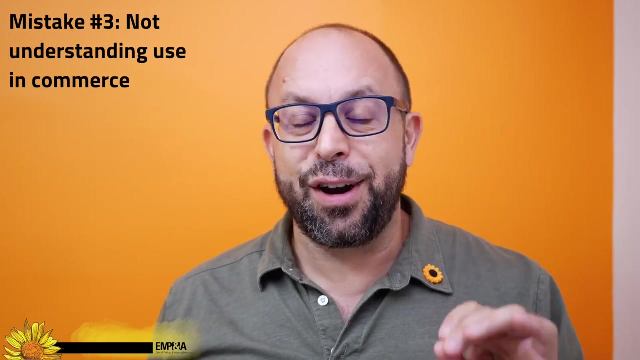 into now A detailed understanding of what use in commerce is. what type of sales qualify for use in commerce and what type of evidence is acceptable to demonstrate use in commerce is a series of highly specialized and sometimes complicated questions. So the fix here is to make sure that you have a good understanding of what use in commerce. 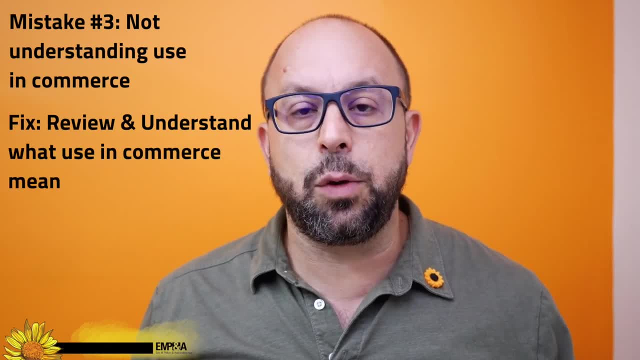 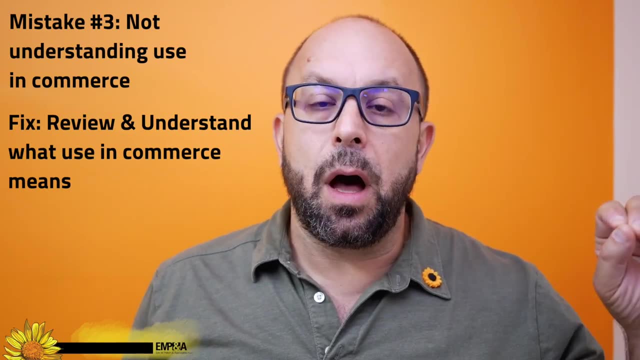 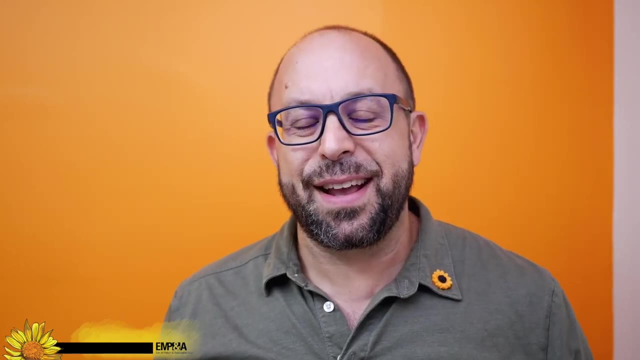 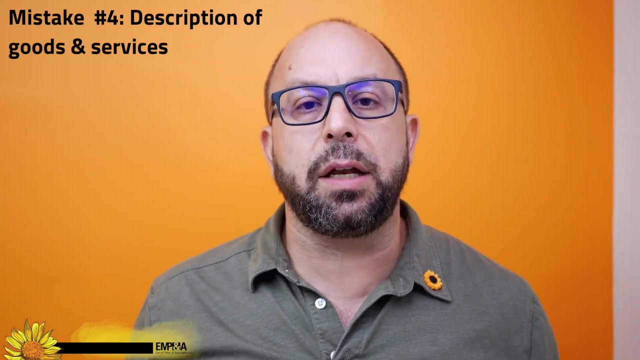 is and what type of evidence is acceptable, and the link between the goods or services in the application and the use and the evidence. The fourth mistake that we often see relates to the description of goods and services. I just mentioned that the use has to be tied to that description of goods and services. 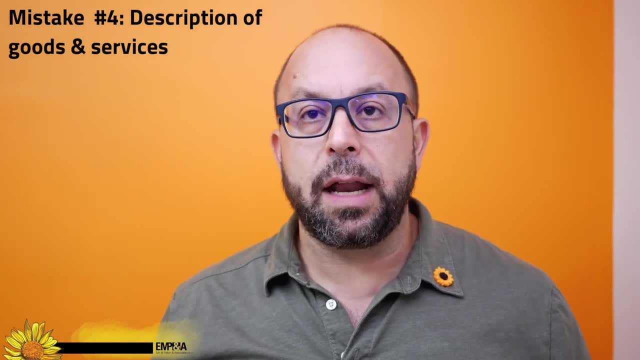 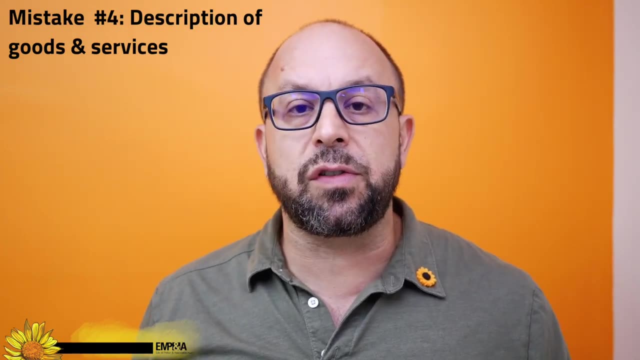 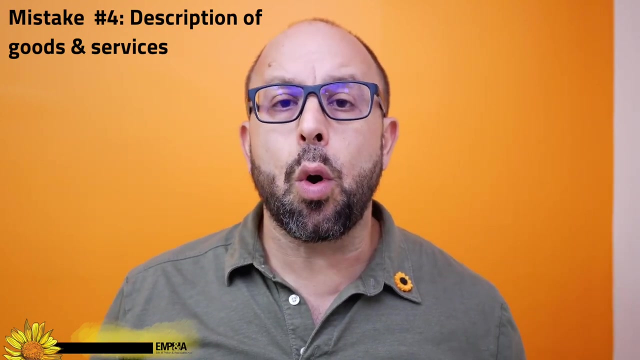 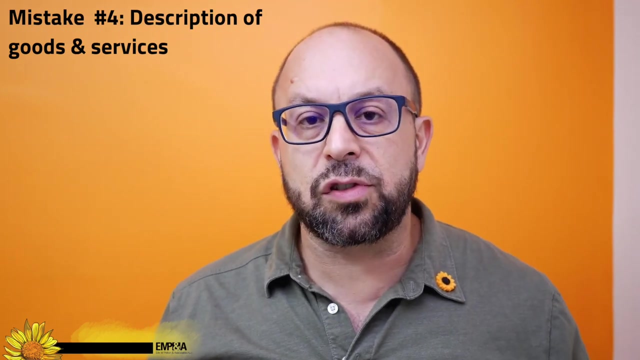 So having a proper and thorough And useful description of goods and services is important. An application might be approved, but if the goods and services description is wrong, such that no evidence of use will be available, the application is no good. Or if crafting the goods and services description differently could lower the risk of a conflict. 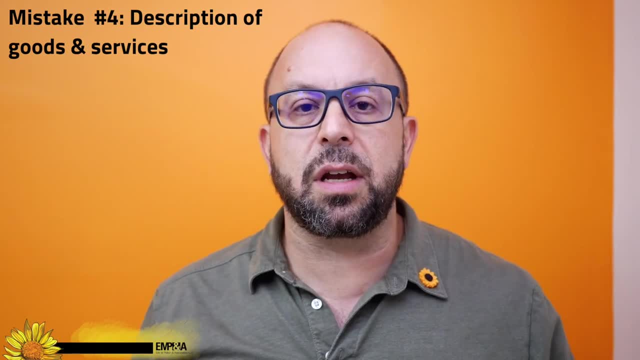 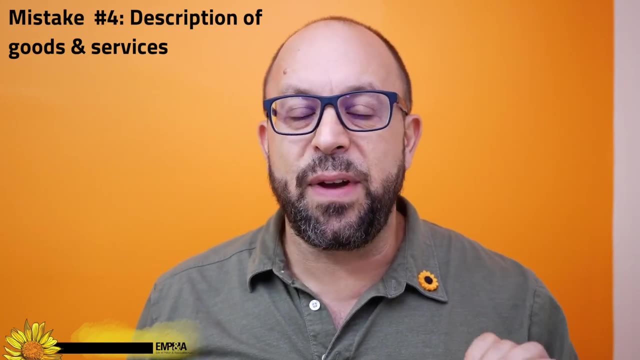 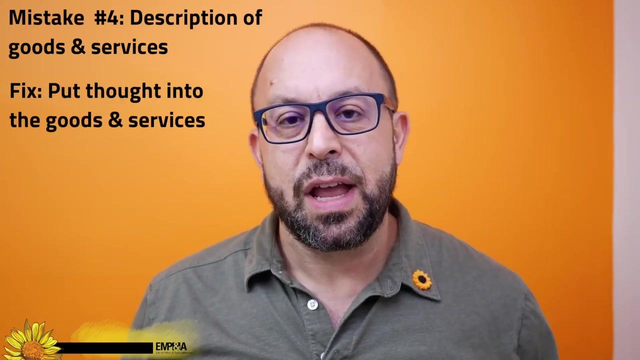 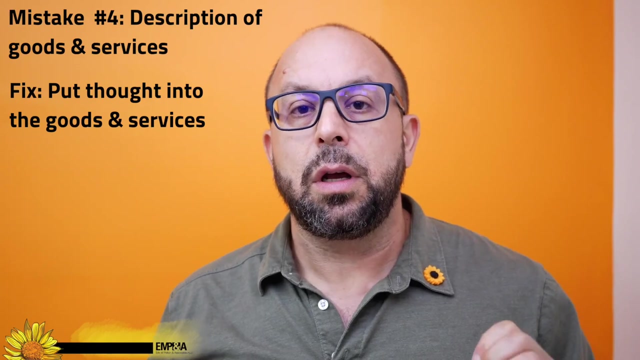 or an issue with the application. that is an important strategic factor to go into drafting and prosecuting the application. So the fix here is to make sure that you put thought into the goods and services and how broad or how narrow or how many classes are chosen to go into the application. 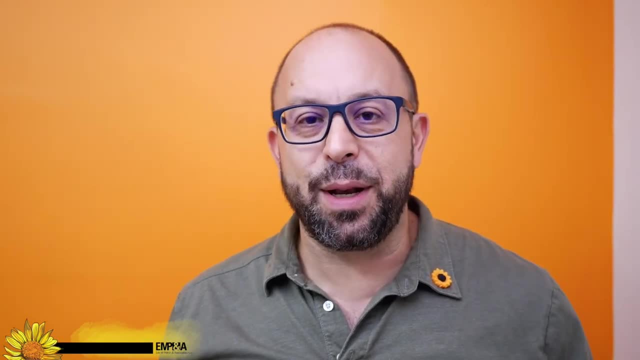 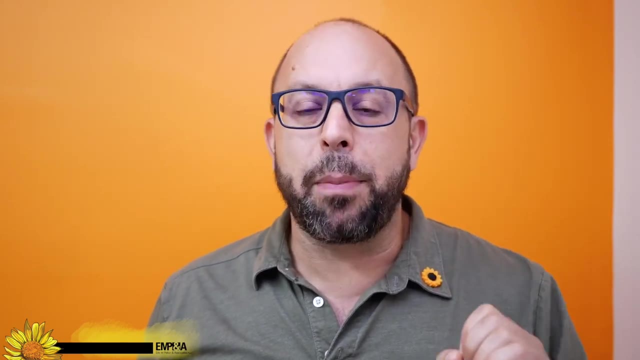 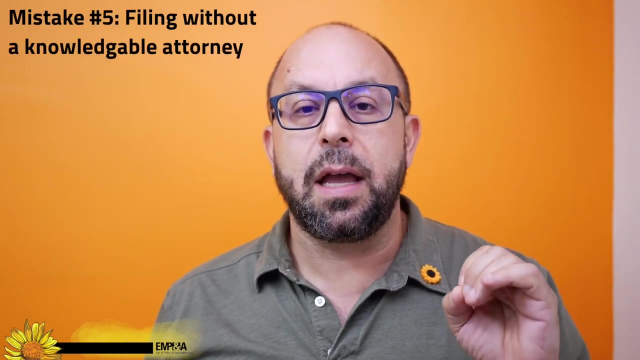 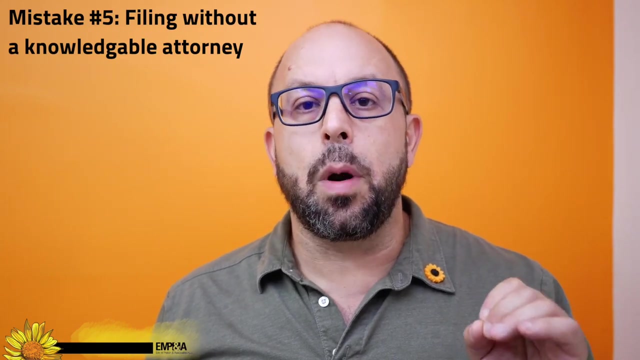 And finally, the fifth very common mistake that I often see actually relates to all four of the other services, And it's probably no big surprise that I'm going to tell you that filing without an attorney, without a knowledgeable experience guide to help through the trademark application process, leads to more problems and leads to a lower rate of success in the application. 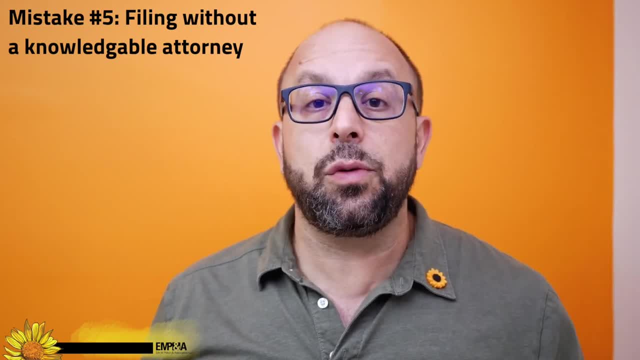 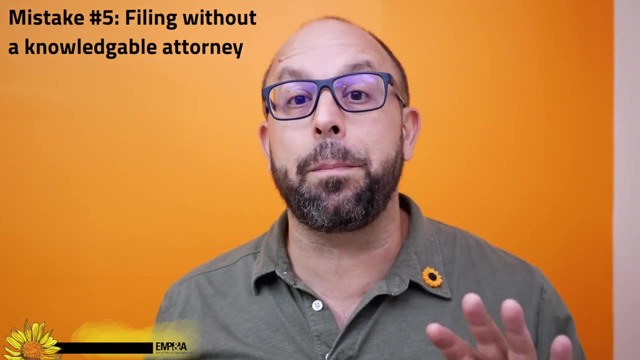 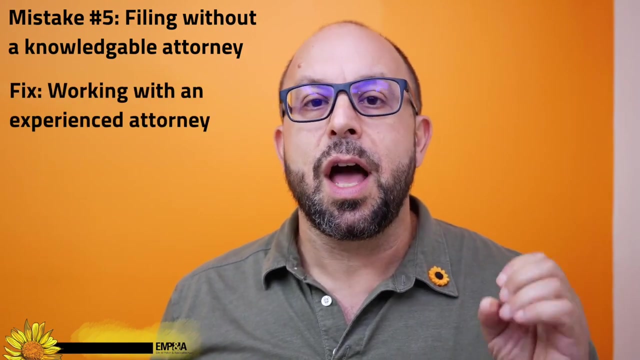 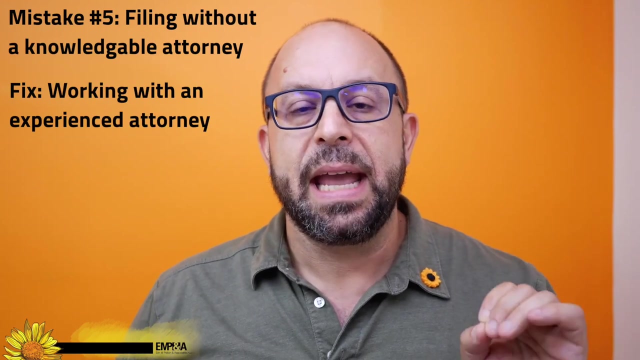 Because, as you've seen, I just mentioned four issues that are complicated, that applicants need to be aware of. There are many, many others as well. Those are just four big, very common ones. So working with experienced counsel is the solution to this problem and to many of the particular problems that can come up in an application.